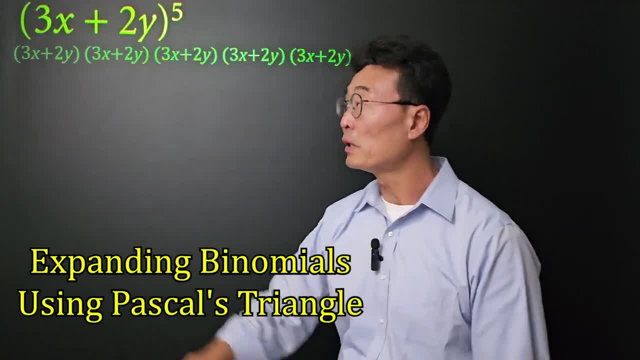 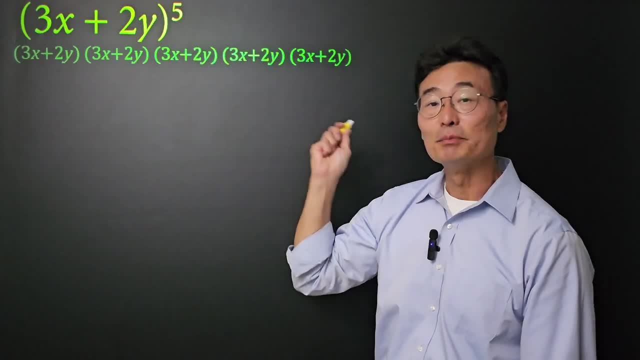 In order to take the binomial 3x plus 2y to the fifth power, you have to multiply 3x plus 2y five times. This could be quite a bit of work. Here's a better way. Let me introduce you to. 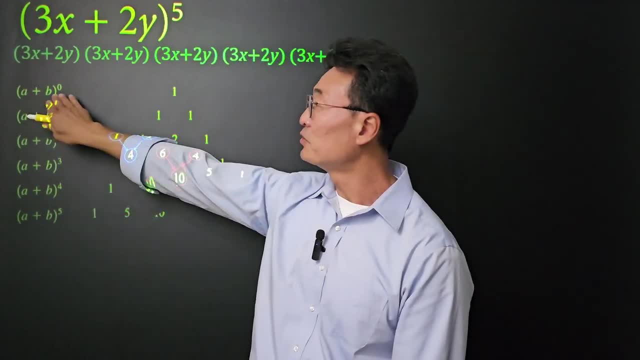 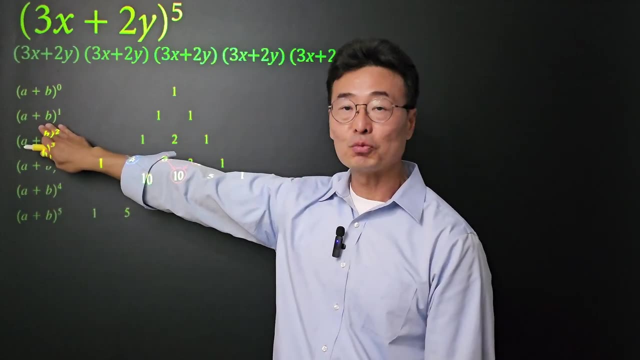 Pascal's triangle. When you have a plus b to the zero power, of course it's going to be one, because anything to the zero power is always one. And then, when we have a plus one to the first power, because the coefficient of a is one and coefficient of b is one, we have one and one. 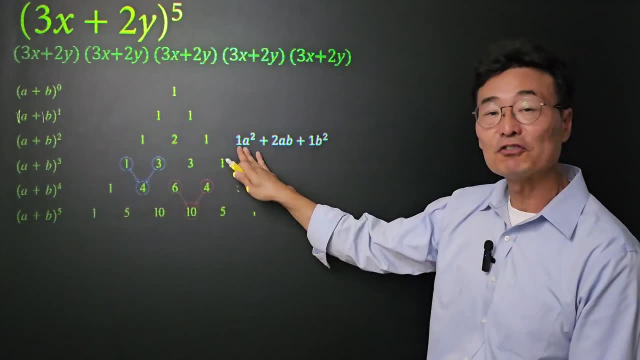 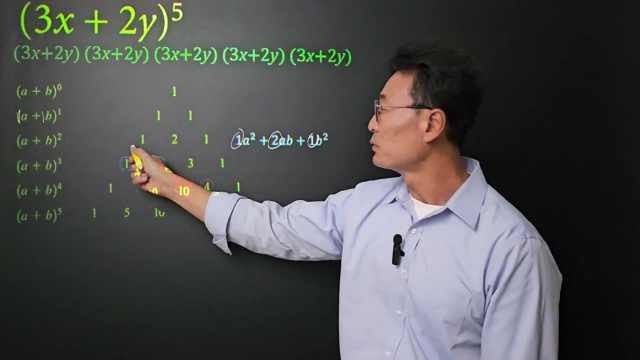 And then when you do a plus b squared, we get one a squared plus two ab plus one b squared. So from the one, two and the one, that's where we get the one, two and the one in the Pascal's triangle. 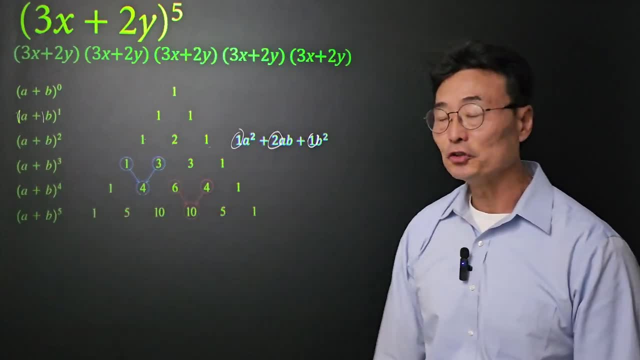 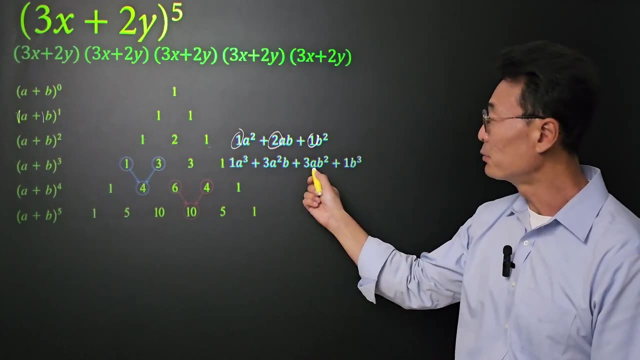 And then one more. If we were to do one plus b to the cube power or to the third power, we get one a cubed plus three a squared, Or b plus three ab squared plus one b cubed. where again the one, three, three and one. 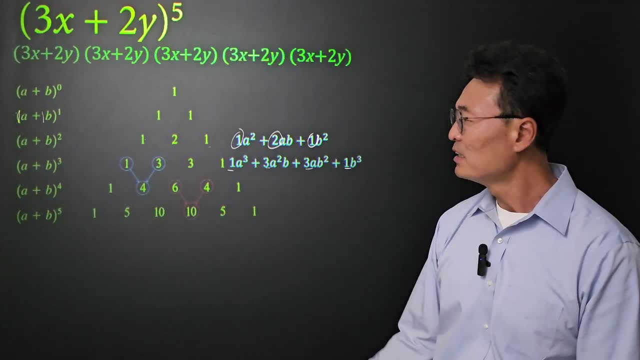 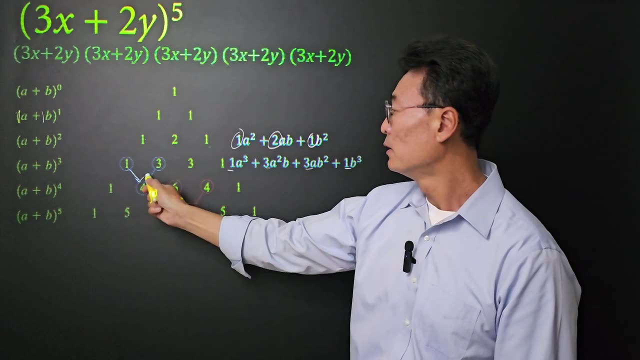 we have it here: one, three, three and one in the Pascal's triangle. So instead of multiplying out a plus b to the fourth power, this is what we want to do. If we take the one and the three, add it up, we get a four, Just like up here, where we added a one. 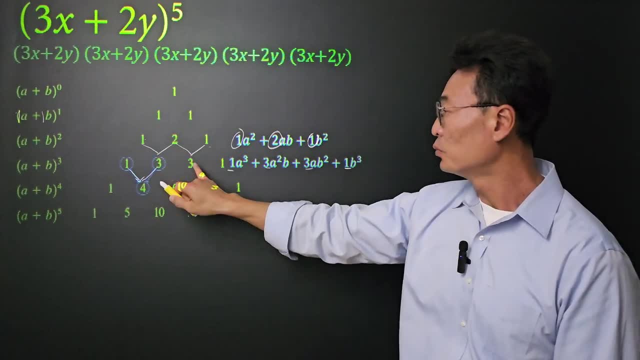 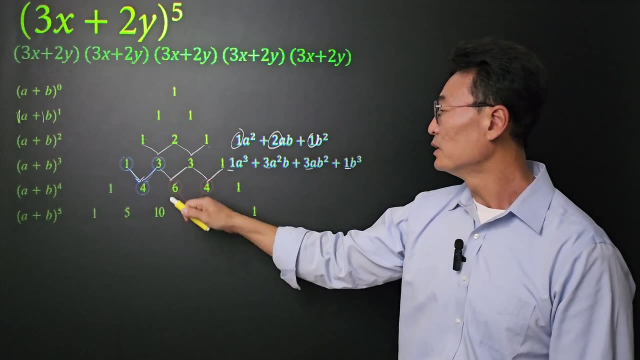 and a two, we got a three. Where we added the two and the one, we got a three again. And then, notice, we get a six, And then the three plus one, we get a four, And then the pattern continues just like. 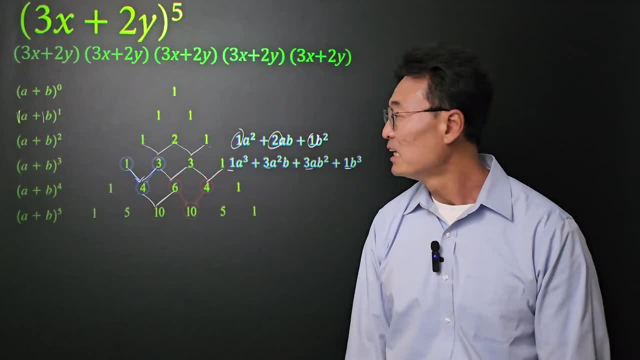 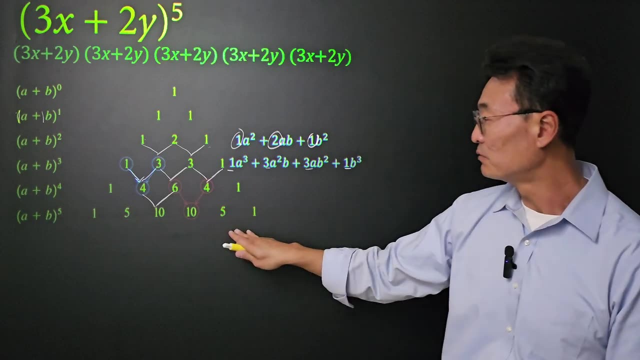 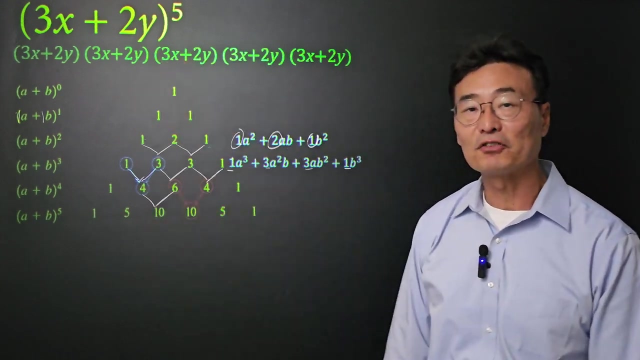 here. If we take the four and the six, we get a ten. Notice that to do a plus b to the fifth power, we have the coefficients of the polynomials here written out already. Then, to apply this to the three x plus two y to the fifth power, here's what we're going to do. We begin by: 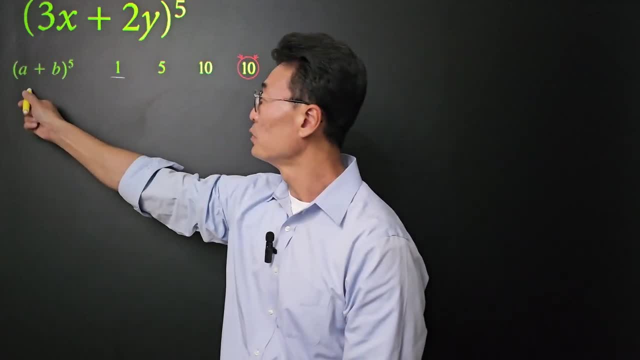 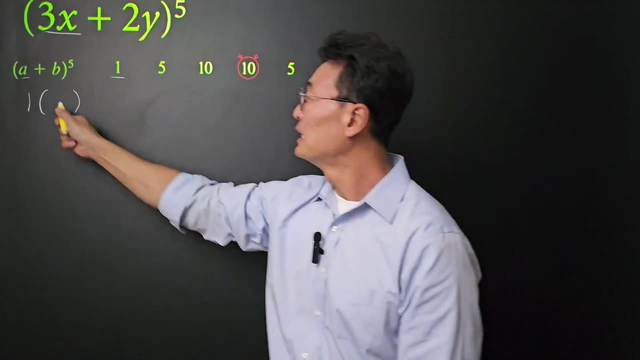 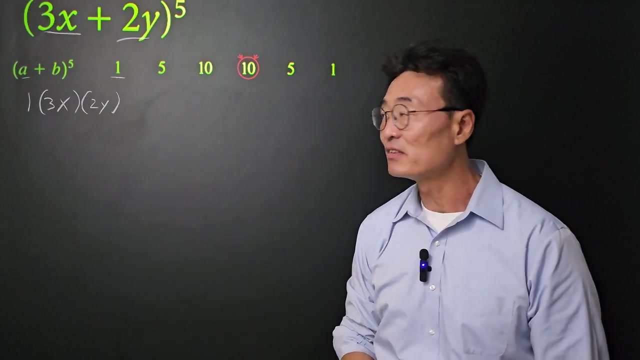 writing the one As the leading coefficient, So it's going to be one, And in parentheses I'm going to write down the three x, which is equivalent of a, or the first of the binomial, in parentheses of course. And then I'm also going to put in the two y in the parentheses as well, which of course is for. 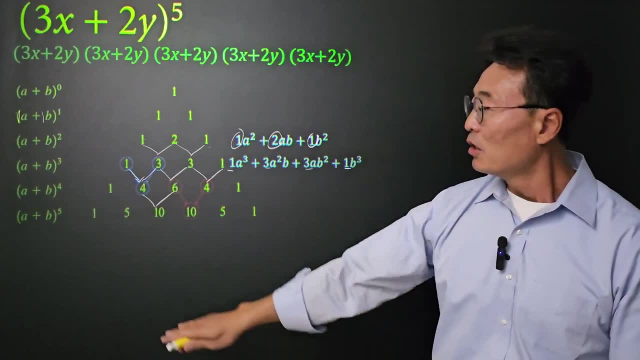 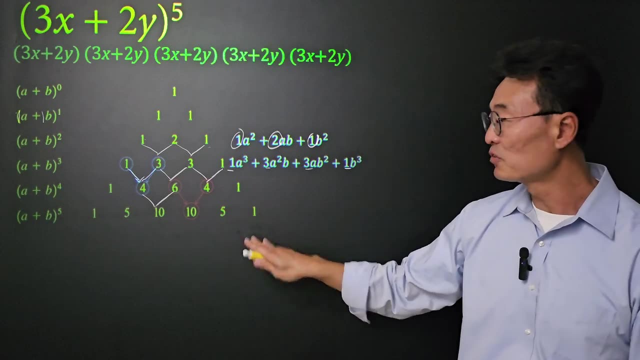 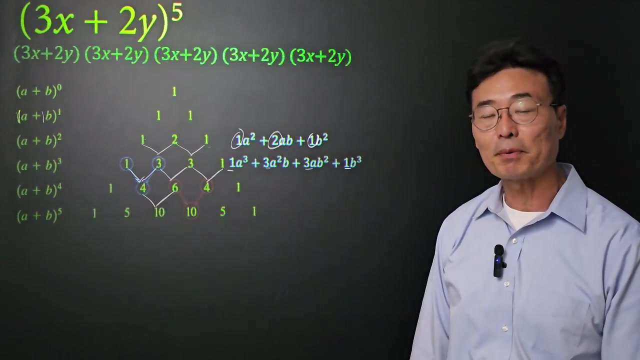 four and the six, we get a ten. Notice that to do a plus b to the fifth power, we have the coefficients of the polynomials here written out already. Then, to apply this to the three x plus two y to the fifth power, here's what we're going to do. We begin by writing the one. 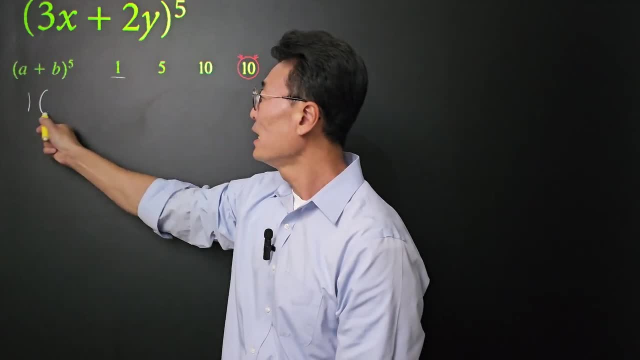 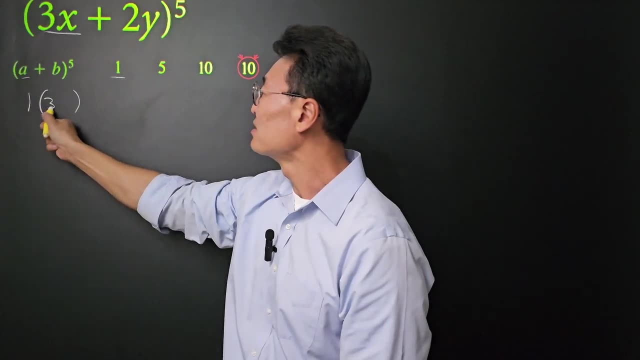 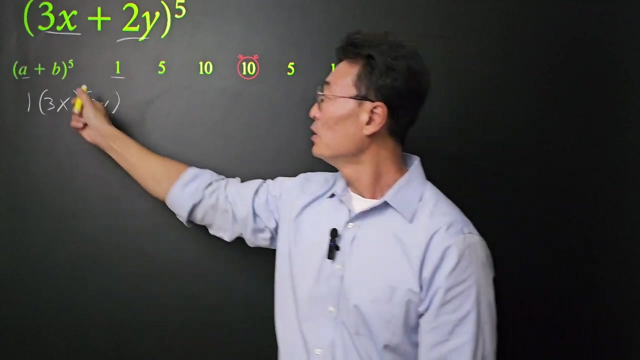 as the leading coefficient. So it's going to be one, And in parentheses I'm going to write down the three x, which is equivalent of a, or the first of the binomial, in parentheses of course. And then I'm also going to put in the two y in the parentheses as well, which of course is for. 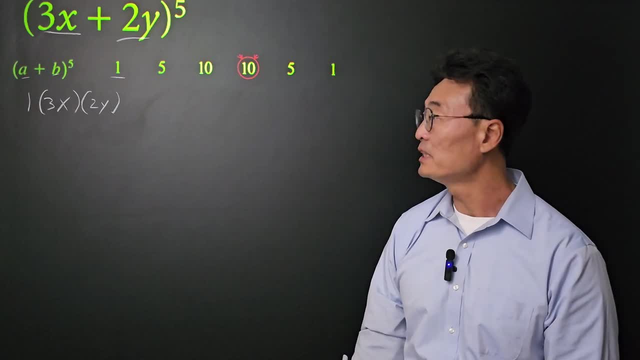 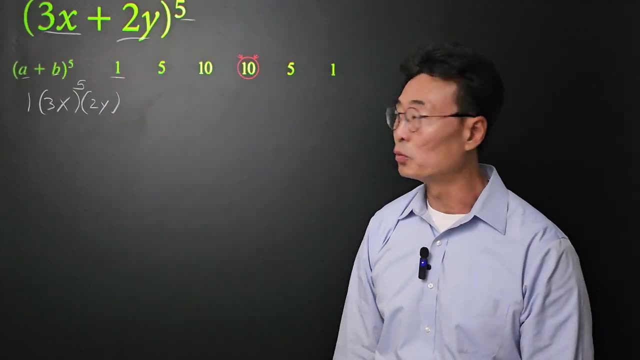 the second binomial, or, in order to replace the letter b, Next the three x: the first one, we'll get the power of five, which is the exponent that we start with, And then the two y gets an exponent of zero, because these two exponents have to add up to. 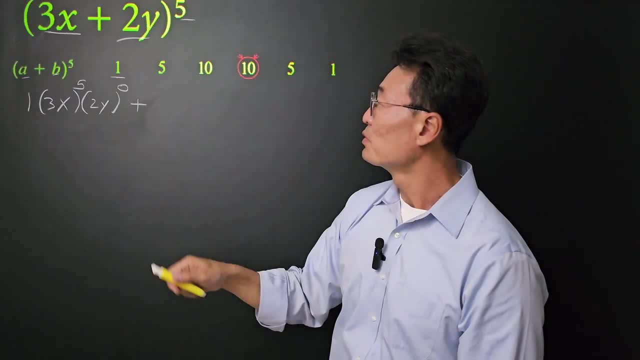 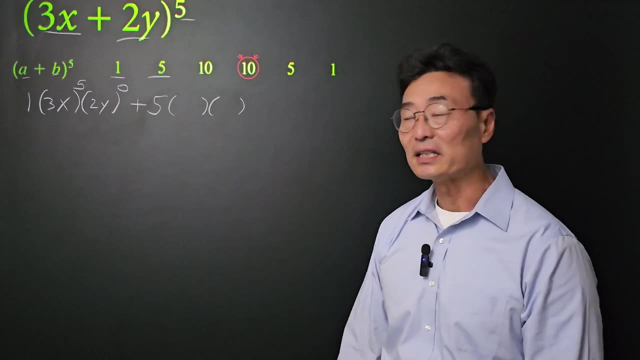 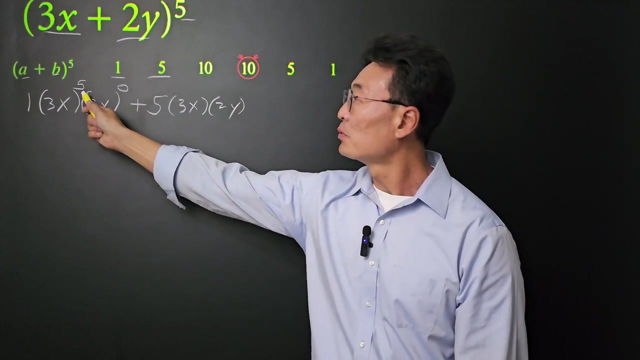 five. That's the pattern. Next plus once again. next coefficient will be five. So I'm going to write down the five And notice the two sets of parentheses I write down first. to start with, I'm going to write down the three x and the two y, And then what happens with the exponent that. 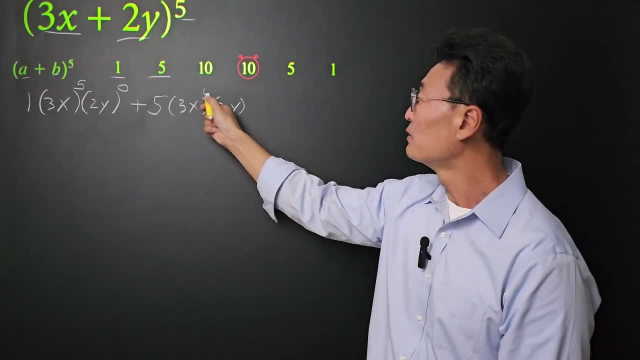 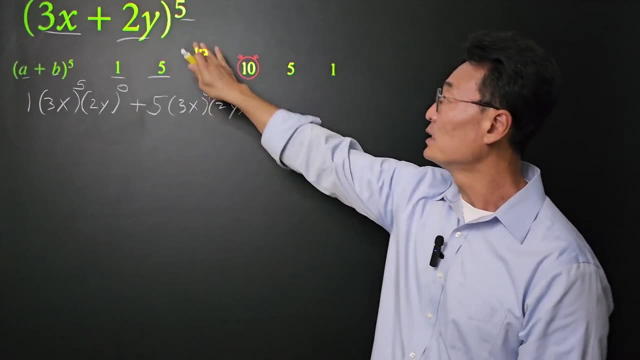 we have. for the three x the five that we have, we go down by one, giving us a four, Whereas zero that we started with it goes up by one, And once again the four and the one adds up to five. 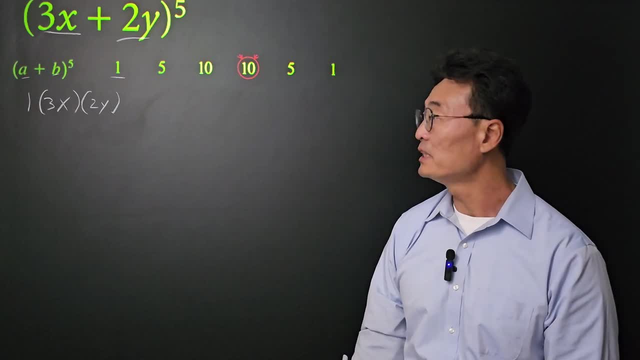 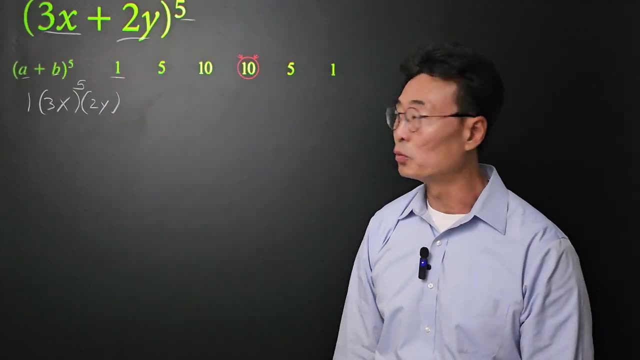 the second binomial, or, in order to replace the letter b, Next the three x: the first one, we'll get the power of five, which is the exponent that we start with, And then the two y gets an exponent of zero, because these two exponents have to add up to. 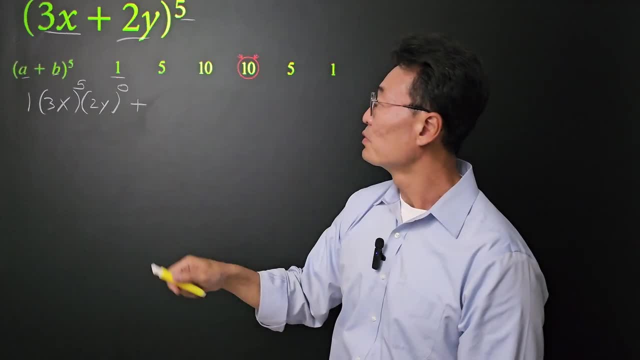 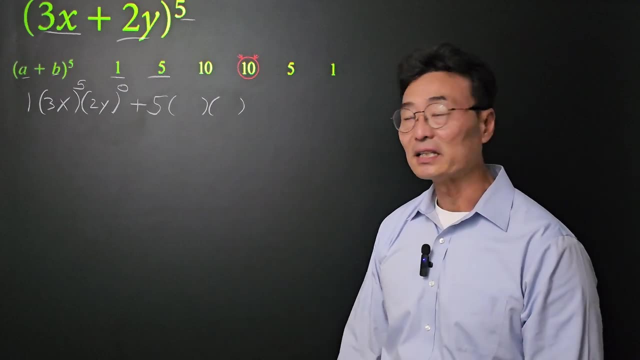 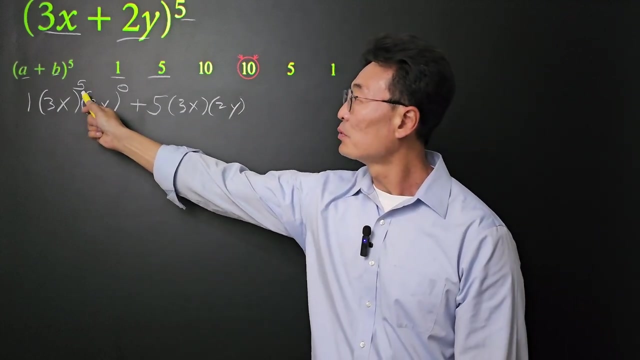 five. That's the pattern. Next plus once again. next coefficient will be five. So I'm going to write down the five And notice the two sets of parentheses I write down first. to start with, I'm going to write down the three x and the two y, And then what happens with the exponent that. 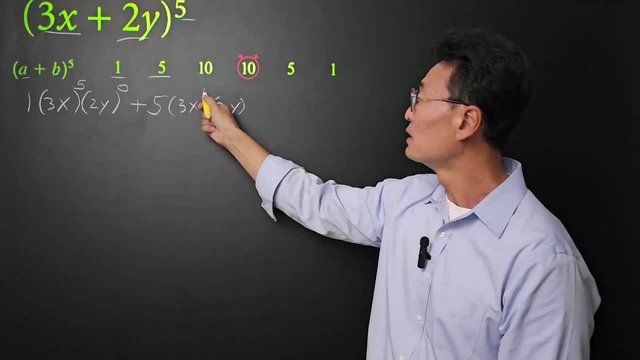 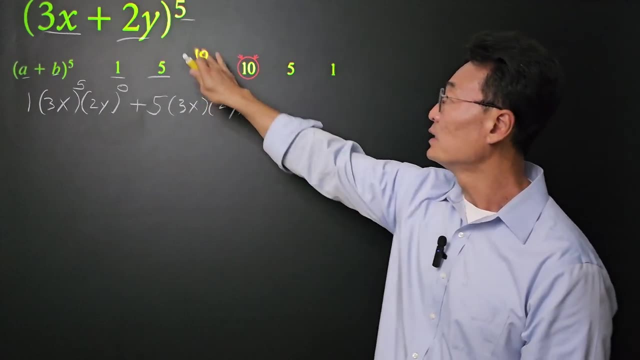 we have. for the three x the five that we have, we go down by one, giving us a four. The zero that we started with it goes up by one And once again the four and the one adds up to five. 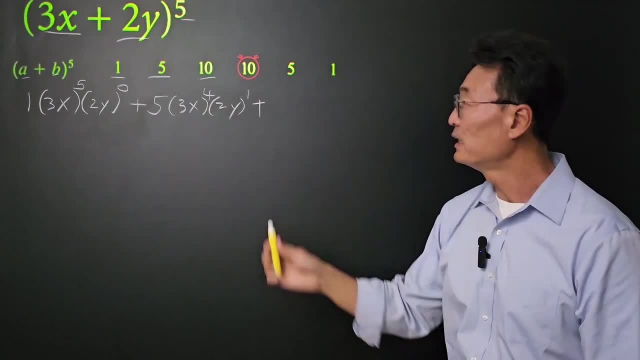 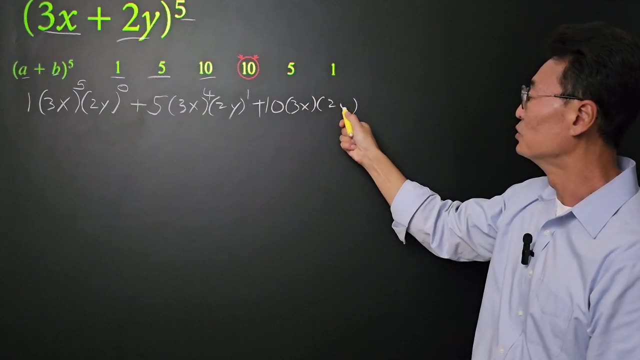 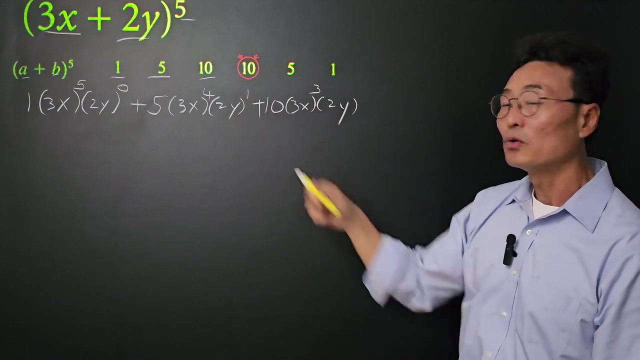 If we continue plus next, coefficient will be ten. Again, write down the two sets of parentheses where we put in the three x and the two y. Again, the four goes down by one where we get a three. Two y goes up by one where we get a two. Next I'm going to continue down here underneath. 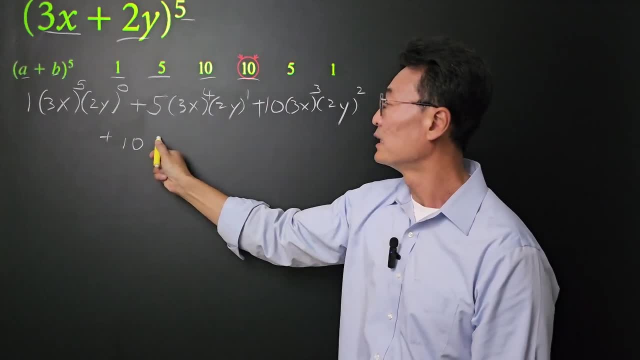 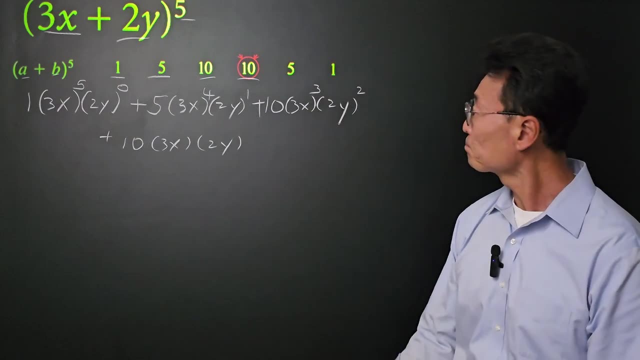 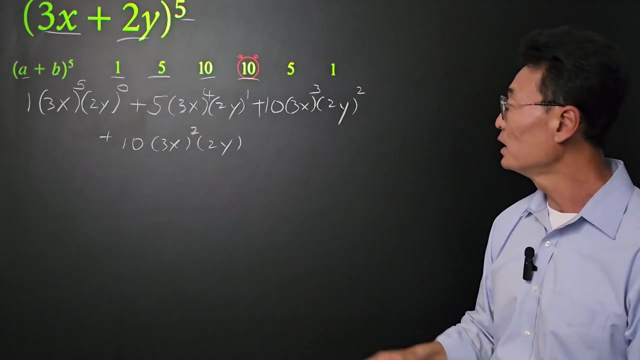 Next coefficient will be ten. So we have our ten Again. notice the two sets of parentheses. I write down Same thing: three x and two y. For the three x we had a cube or three power just now. So we're now going to write down two where we go down by one, Whereas the two goes up by one. 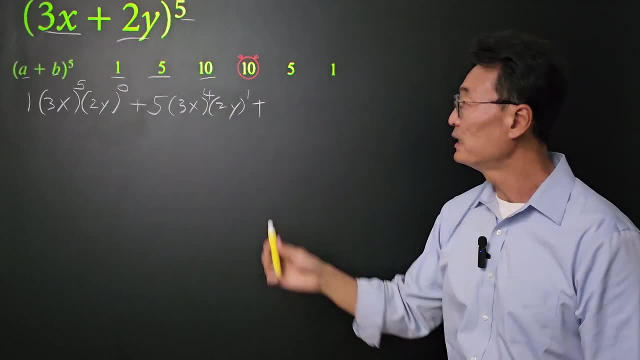 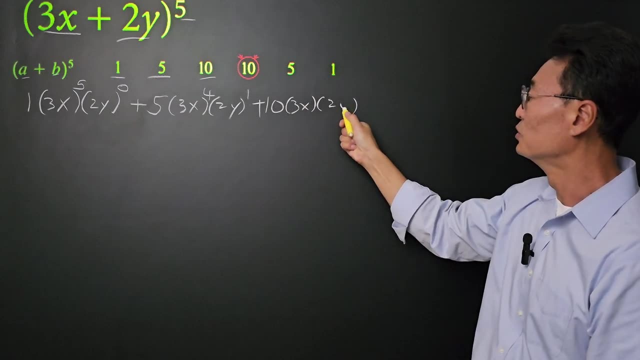 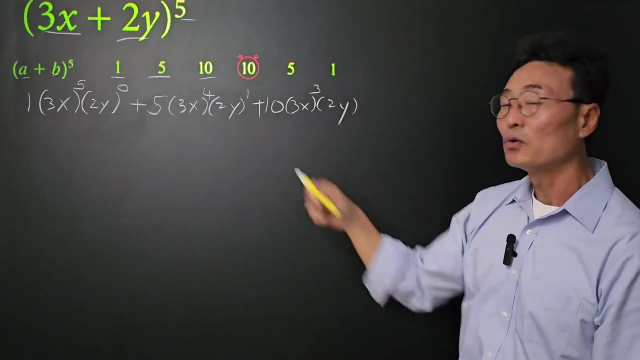 If we continue plus next, coefficient will be ten. Again, write down the two sets of parentheses where we put in the three x and two y. Again, the four goes down by one where we get a three. Two y goes up by one where we get a two. Next I'm going to continue down here underneath. 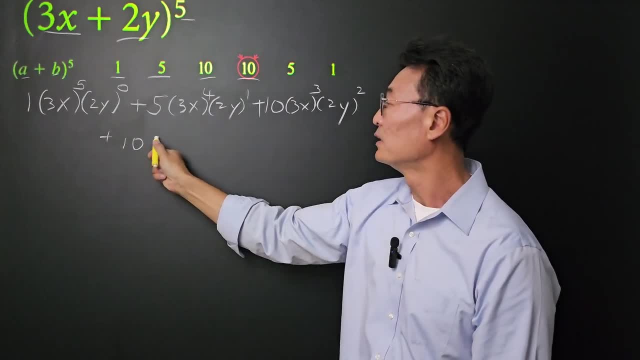 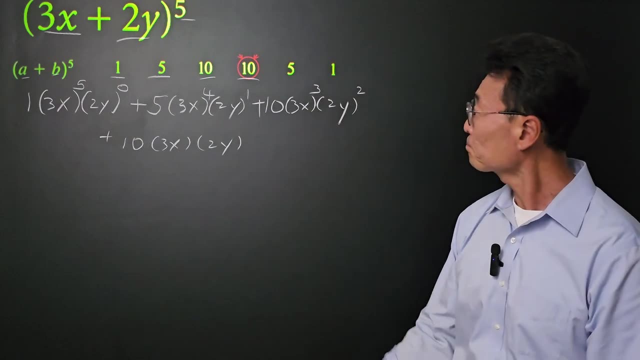 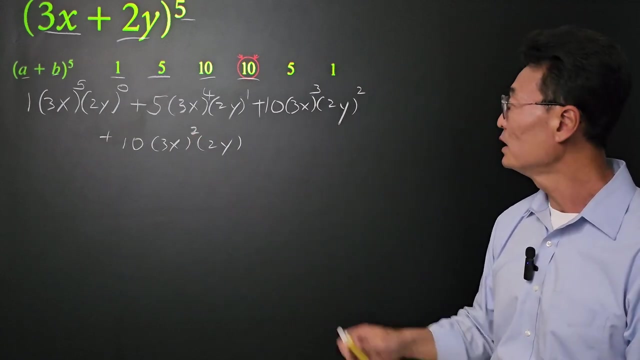 Next coefficient will be ten. So we have our ten Again. notice the two sets of parentheses. I write down Same thing: three x and two y. For the three x we had a cube or three power just now. So we're now going to write down two where we go down by one, Whereas the two goes up by one. 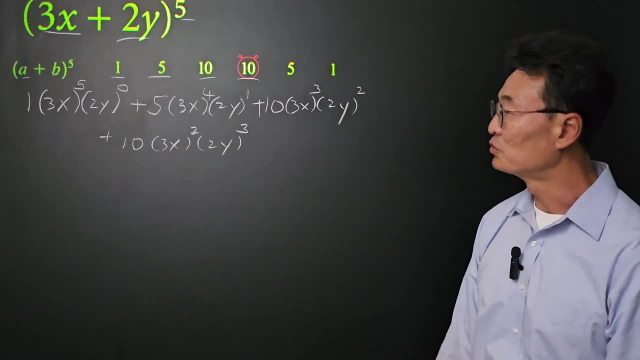 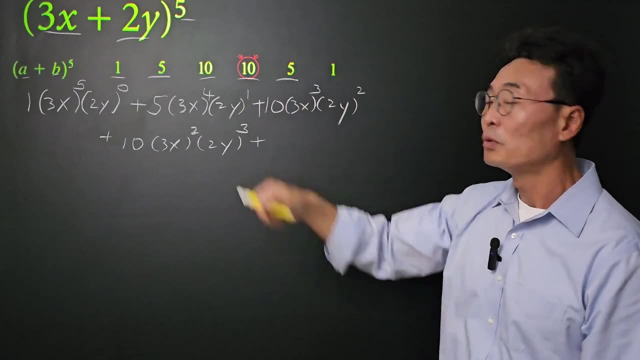 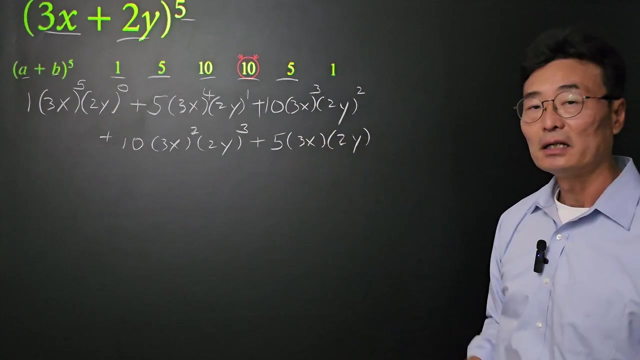 so it becomes a three. And notice, as always, the exponents, the two and the three three and the two four and the one. they all add up to five Plus. we're almost done. Next one will be coefficient of five. Again, I'm going to put three x and two y in the parentheses. 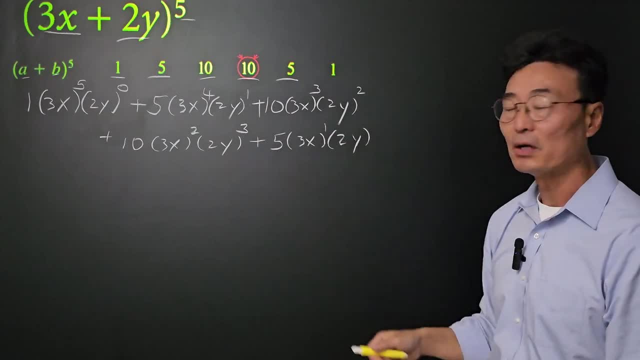 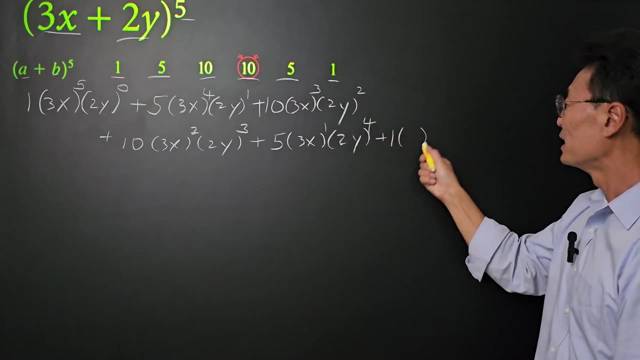 Two goes down by one, so we now have a one. Three goes up by one, so we now have a four Plus the last one has a coefficient of one Same thing. we're going to put the three x and two y. 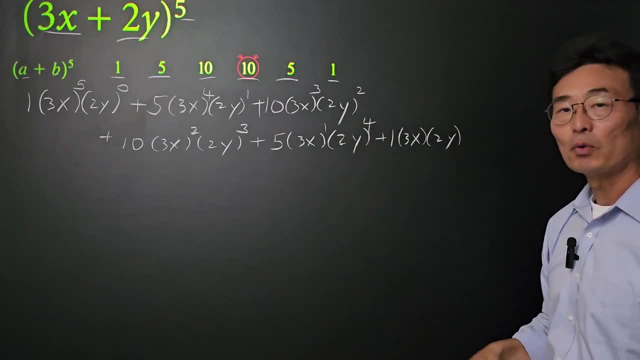 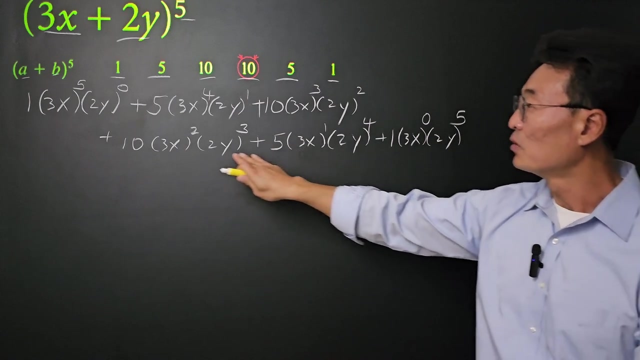 in the two sets of parentheses, And then the one goes down by one, making it a zero, And then the extra one making it a five. There you have it, folks. Only thing left is to go ahead and simplify the coefficients, along with the coefficient of the variables, Along with the exponents. 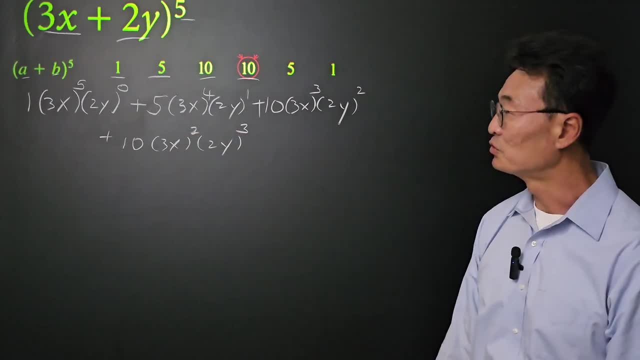 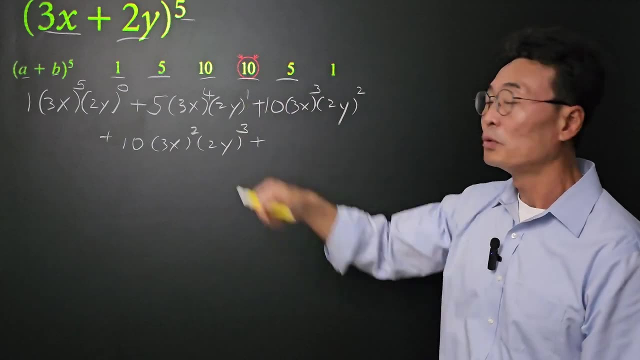 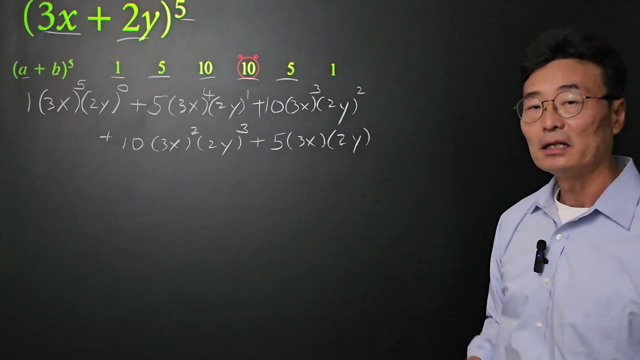 so it becomes a three. And notice, as always, the exponents, the two and the three three and the two four and the one. they all add up to five Plus. we're almost done. Next one will be coefficient of five. Again, I'm going to put three x and two y in the parentheses. 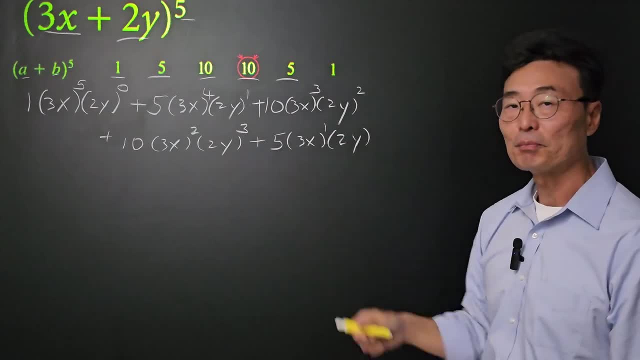 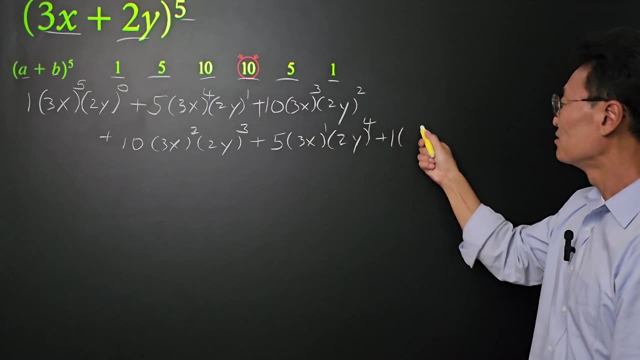 Two goes down by one, so we now have a one. Three goes up by one, so we now have a four Plus the last one has a coefficient of one Same thing. we're going to put the three x and two y. 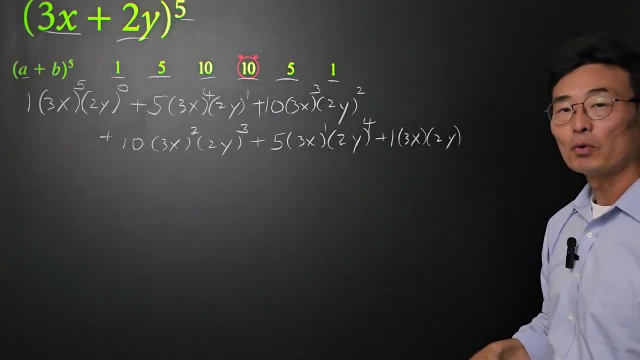 in the two sets of parentheses, And then the one goes down by one, making it a zero, And then the four goes up by one, And then the three x and two y into the one, making it a five. There you have it, folks. Only thing left is to go ahead and simplify. 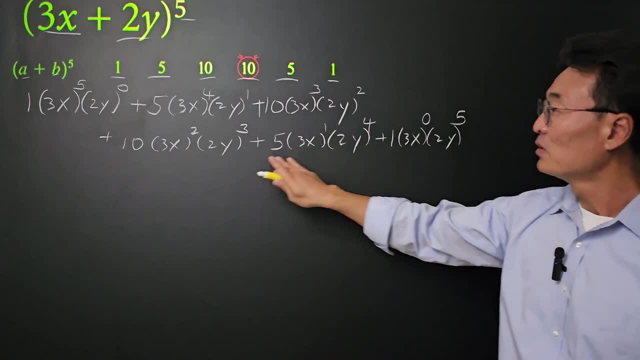 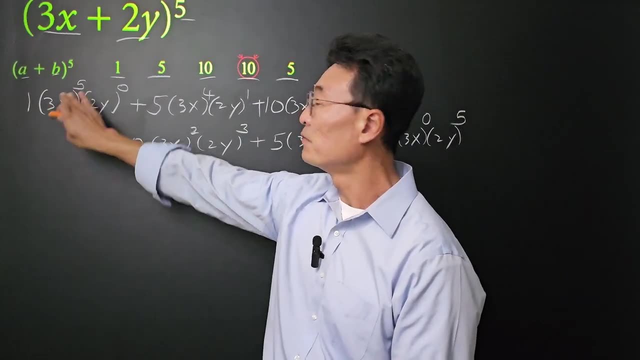 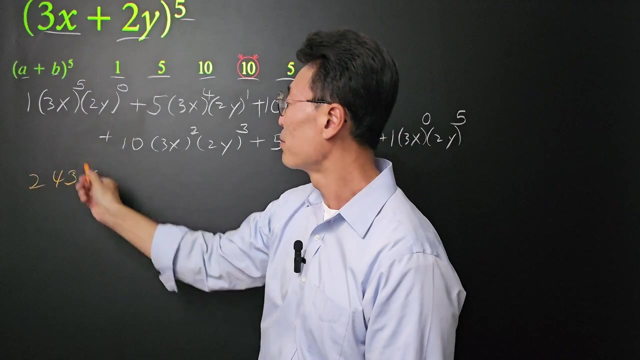 the coefficients, along with the coefficient of the variables, along with the exponents Which I'm gonna show you next. First, we have to the fifth power, which is going to be two-fortych-three: x to the fifth power And two-y to the zero. power is just one, so we could just go ahead and Personalize. 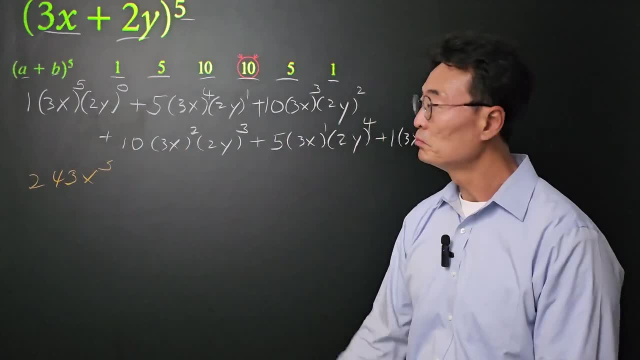 ix to the fifth power and 2y to the zero power is just one And 2y to the zero power is just one. We could just go ahead and simplify: x to the fifth power And 2y to the zero power is just one. 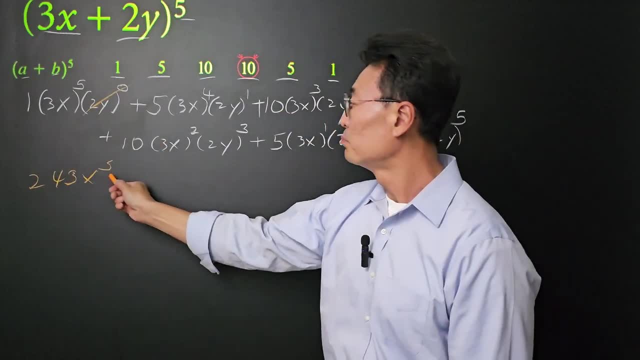 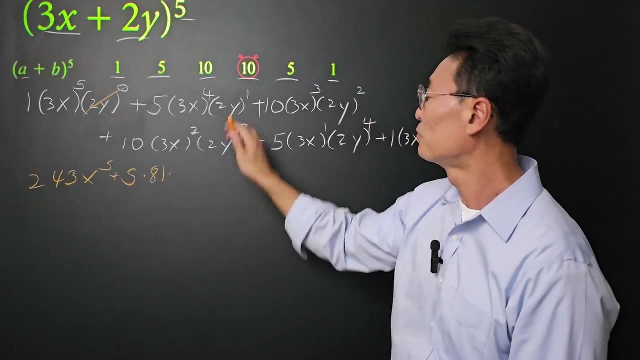 So we could go ahead and simplify first power. So if i hot black, we're gonna go back toểu to the second one, going to cancel that out. And we have plus 5 times 3 to the 4th. power is 81 times 2 to the 1st power. 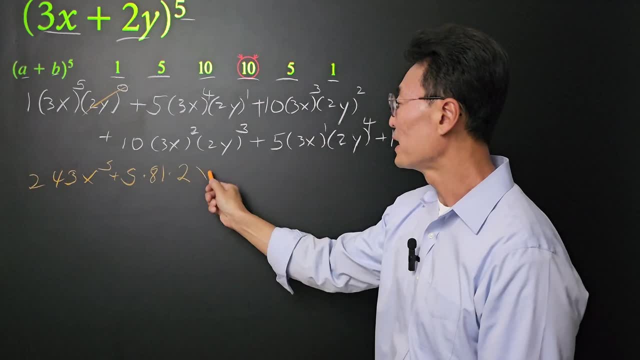 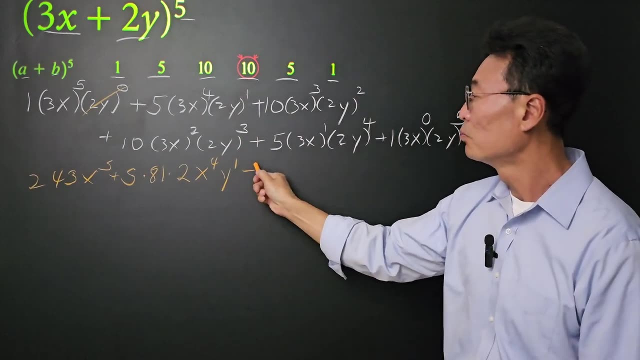 is 2.. And then we got to take care of the x and the y, where we get x to the 4th power from here and y to the 1st power from here, Continuing. plus we have the 10 in the front, 3 to the 3rd. 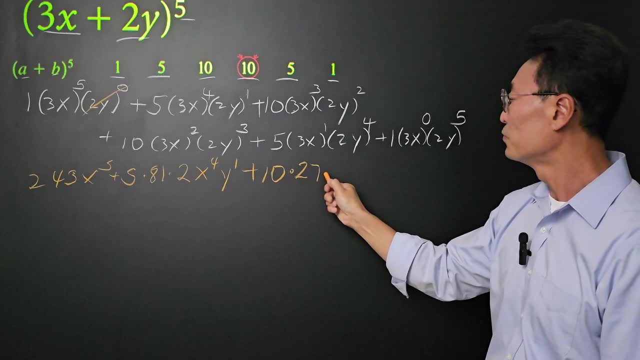 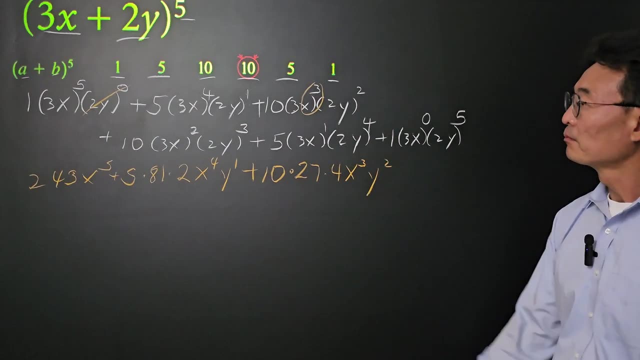 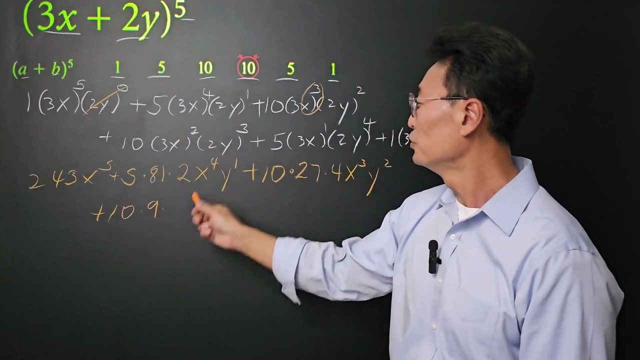 power is 27,. 2 squared is 4, and we have x cubed from here and y squared. Continuing here, once again we have the 10,, 3 squared is 9,, 2 cubed is 8, and we have x squared and y cubed Once again. 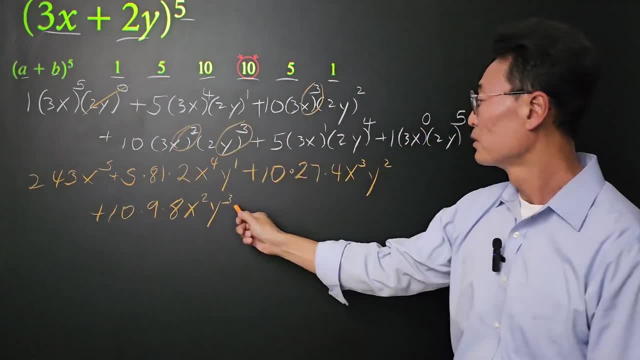 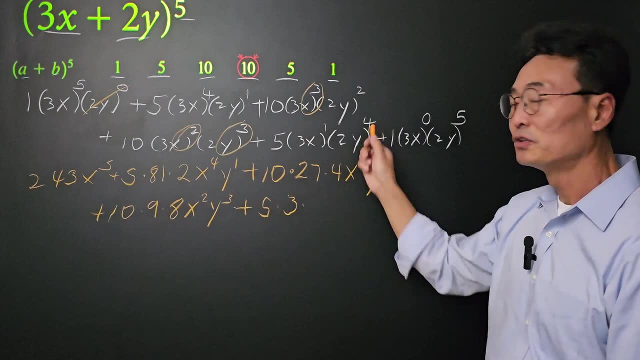 here's our x squared, here's the y cubed. plus we have the 5 to start with and then 3, the 1st power, of course, is 3,. 2 to the 4th is 16,. we have x and y to the 4th, again from here. 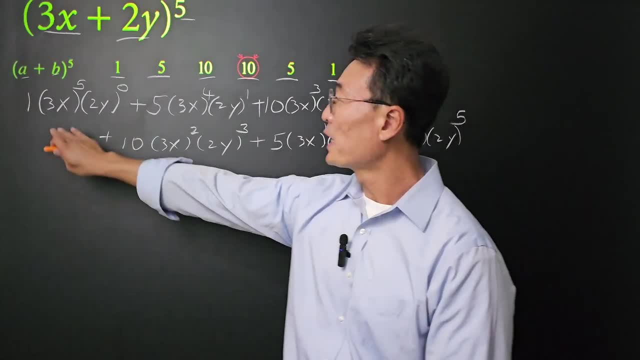 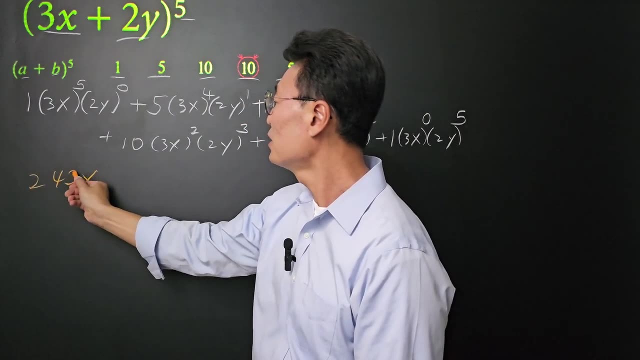 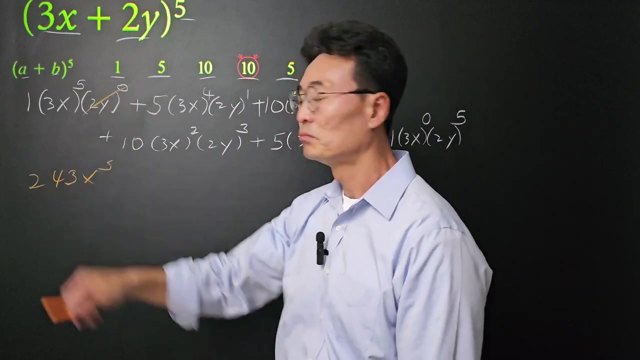 which I'm going to show you next. First, we have 3 to the fifth power, which is going to 243. x to the fifth power And two y to the zero. power is just one, so we can just go ahead and cancel that out and we have plus five times three to the fourth power. 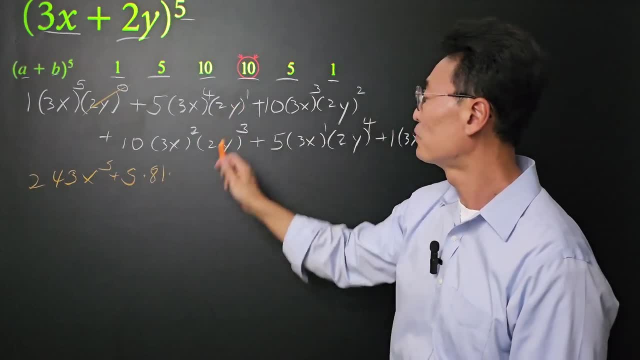 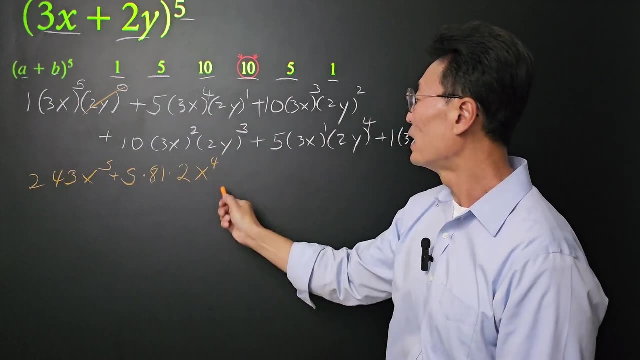 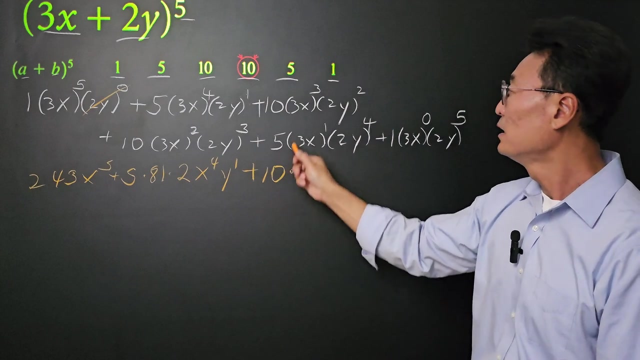 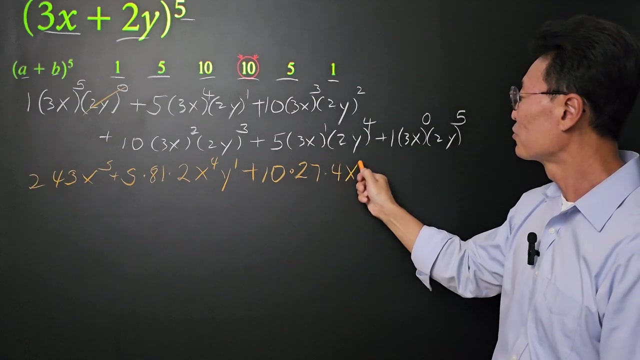 is 81 times two to the first power is two, and then we got to take care of the x and the y, where we get x to the fourth power from here and y to the first power from here, continuing. plus we have a 10 in the front. three to the third power is 27, two square is four and we have x cube from here. 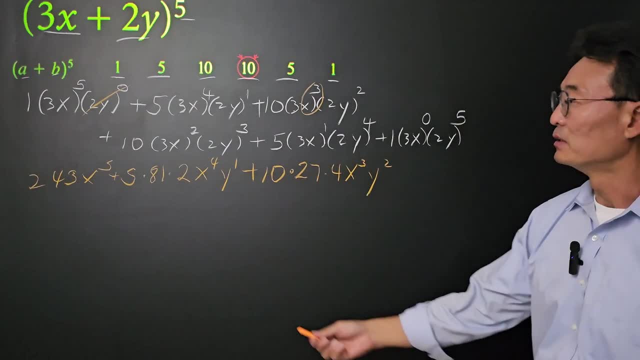 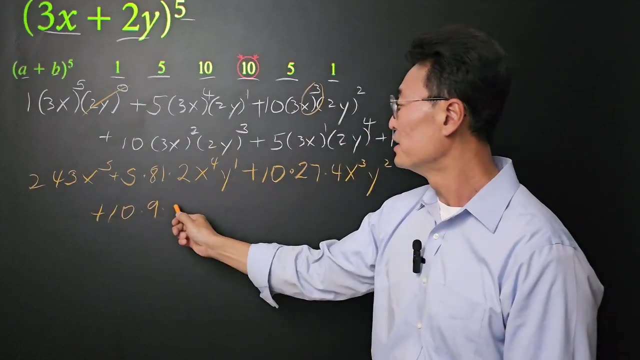 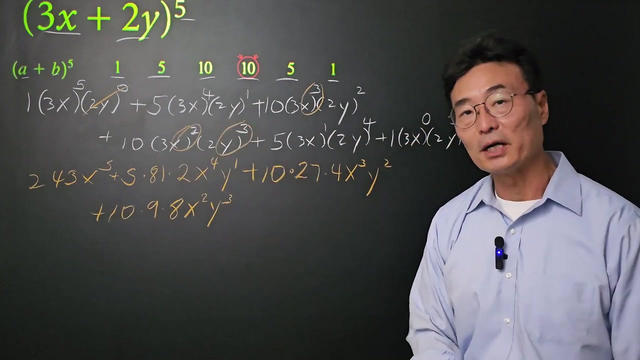 and y square. continuing here, once again we have a 10. three square is nine, two cube is eight and we have x square and y cube. once again, here's our x square, here's the y cube plus. we have the five to start with and then three to the first. power, of course, is three. 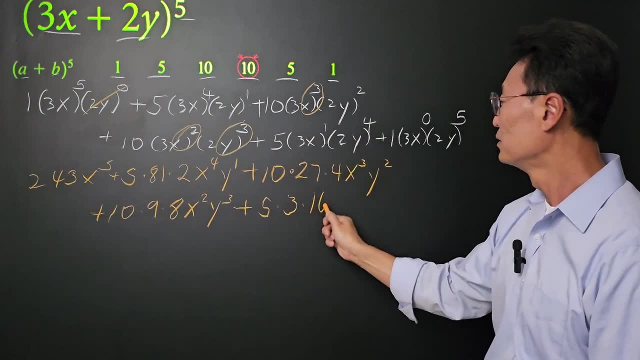 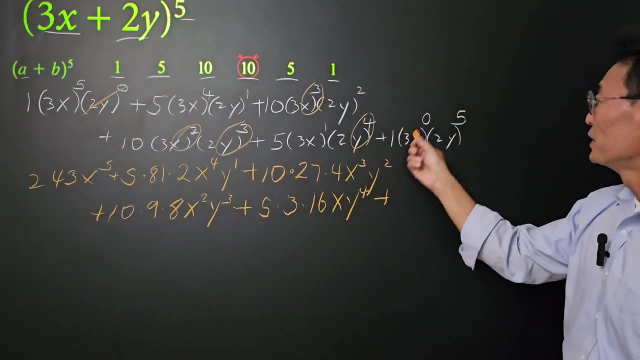 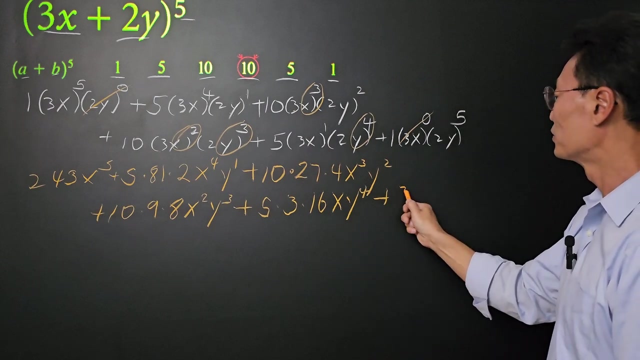 two to the fourth is 16. we have x and y to the fourth, again from here plus three to the zero power, again is one, so we're not worried about that. two to the fifth power is equal to 32, and then we have y to the once again fifth power. 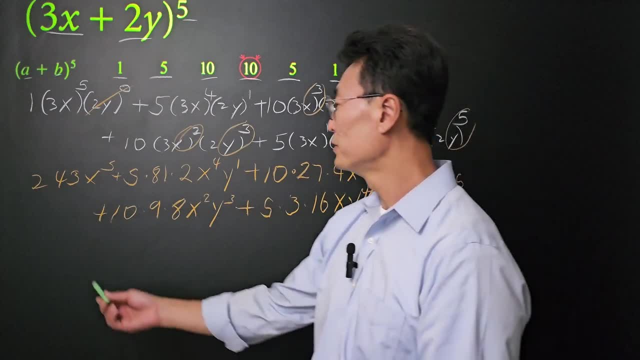 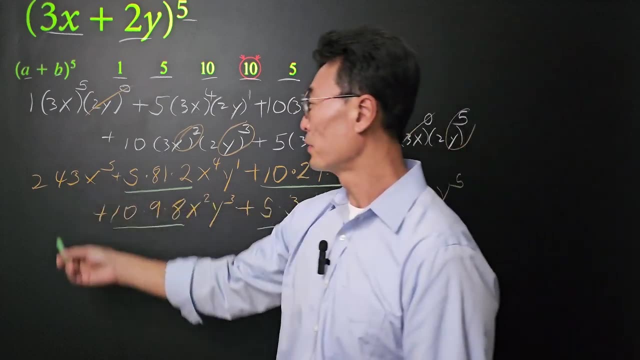 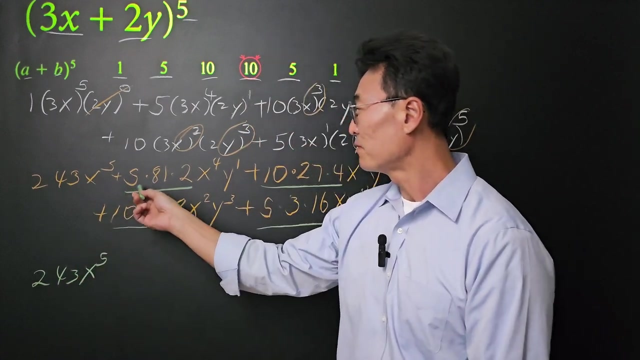 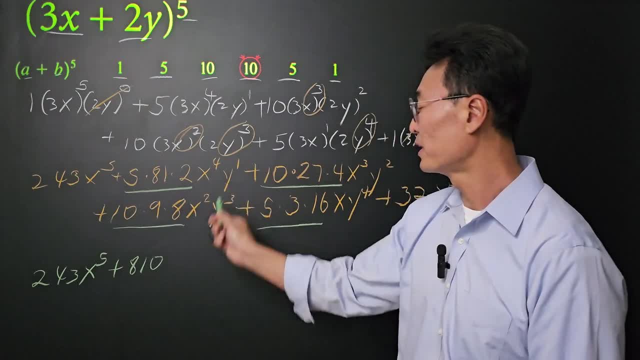 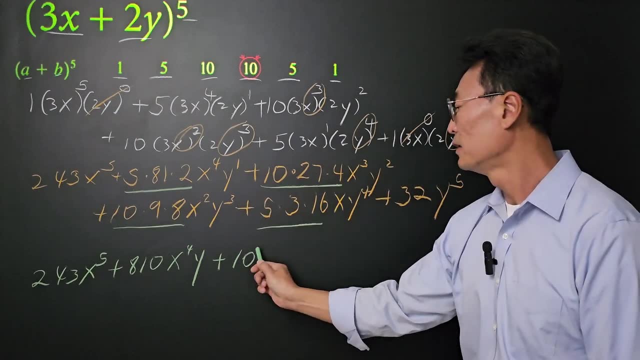 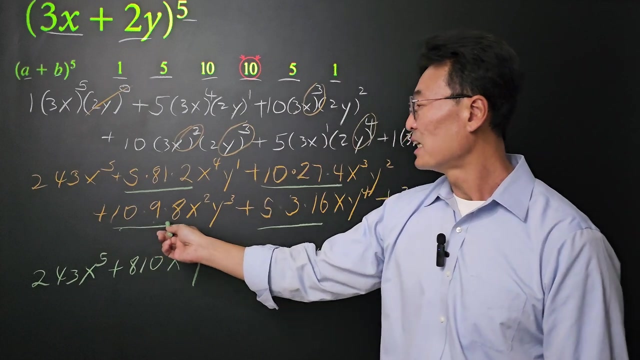 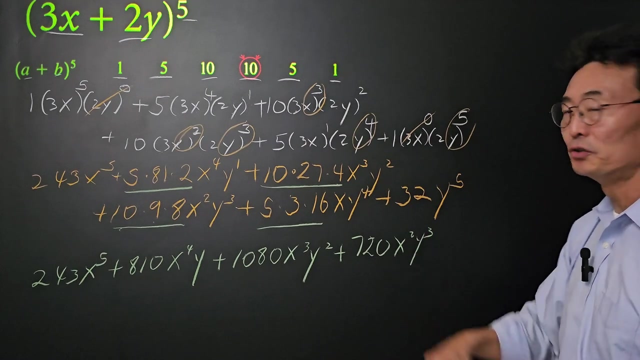 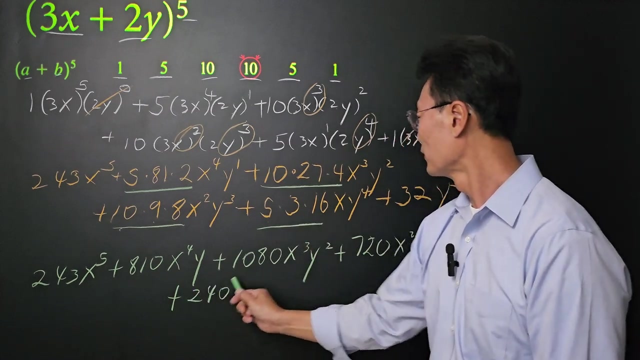 eight ten and again we have our x to the fourth and y plus 10 times 27 times four is 10, 80. and again we have x cube, y square 10 times 9 times 8 is going to be 720. again we have x square and y cube plus 5 times 3 times 16 is 240. 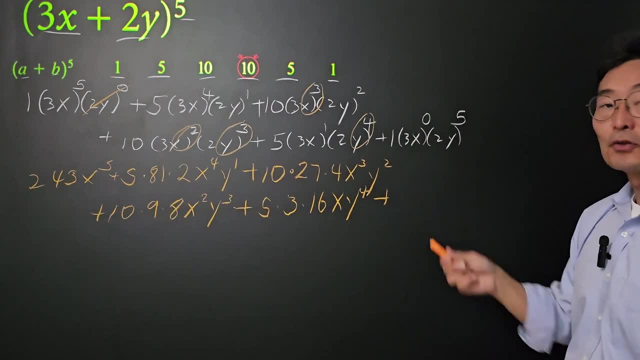 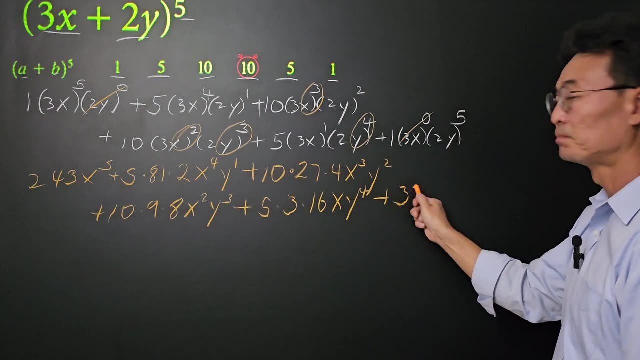 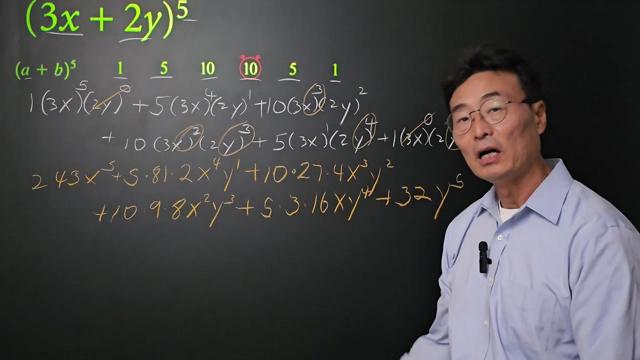 plus 3 to the 0 power again is 1, so we don't have to worry about that. 2 to the 5th power is equal to 32, and then we have y to the once again 5th power. To finish, all we have to do. is go ahead and simplify this, So we have x squared and y cubed, and then we have y to the once again 5th power. To finish, all we have to do is go ahead and simplify this, So we have. 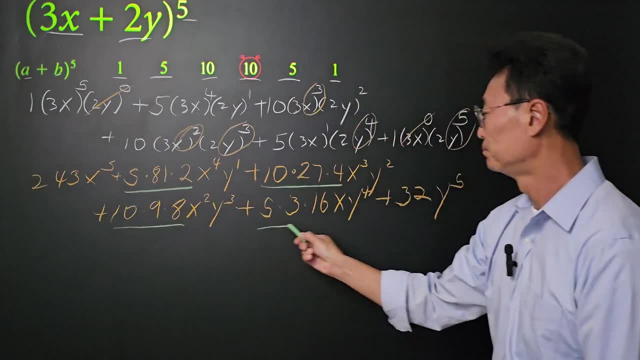 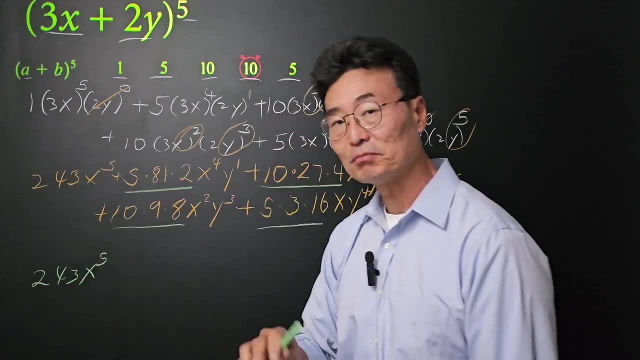 x squared and y cubed, and then we have x squared and y cubed, and then we have y squared, or multiply out the coefficients in the front, First the 243x cubed, or x to the 5th power. that is, nothing changes there. Here we have 5 times 81 times 2,. 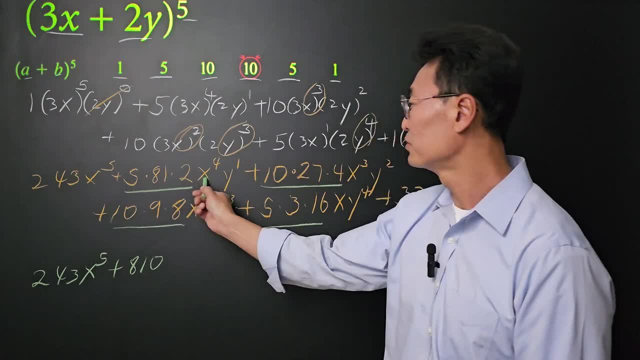 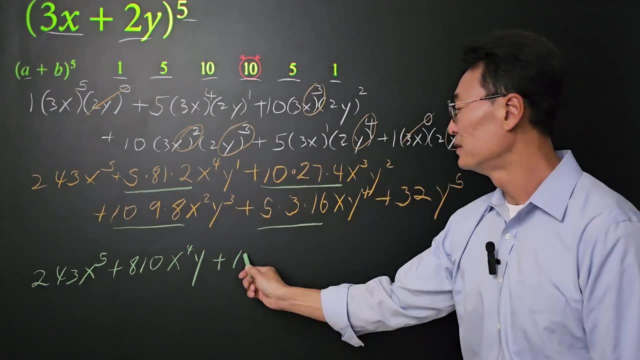 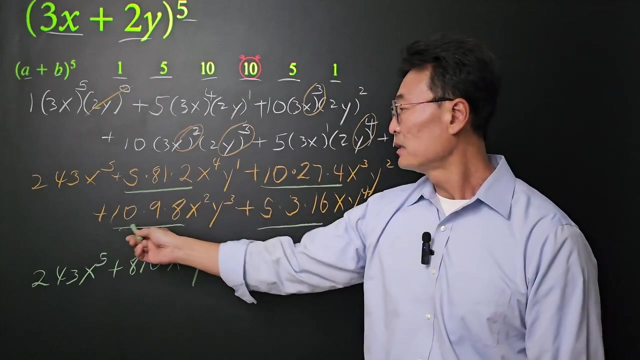 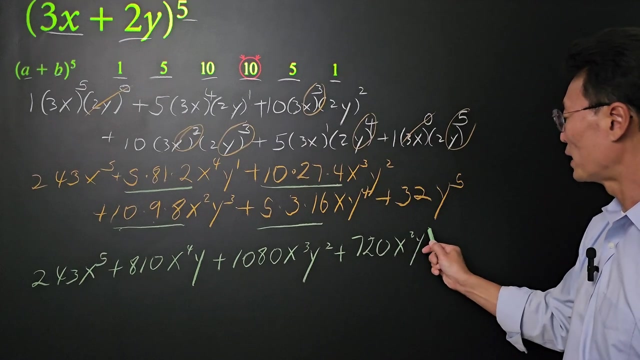 we get 810, and again we have our x to the 4th and y plus. 10 times 27 times 4 is 1080, and again we have x cubed y squared there, 10 times 9 times 8 is going to be 720.. Again we have x squared and y cubed plus. 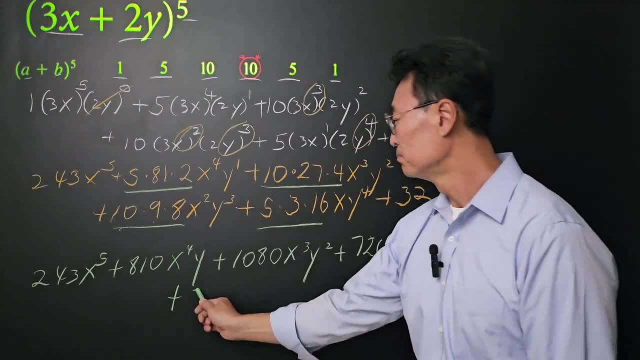 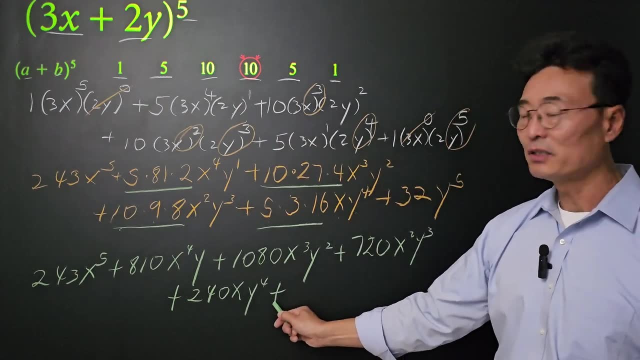 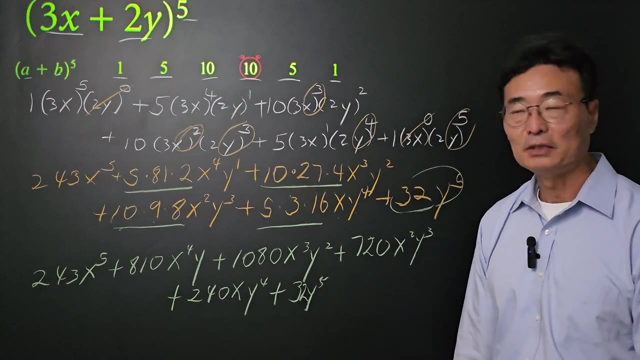 5 times 3 times 16 is 240. Again x and y to the 4th, plus finally we have our 32, y to the 5th power, y to the 1st power is one quarter of the original power realised by a constant. So this solve. 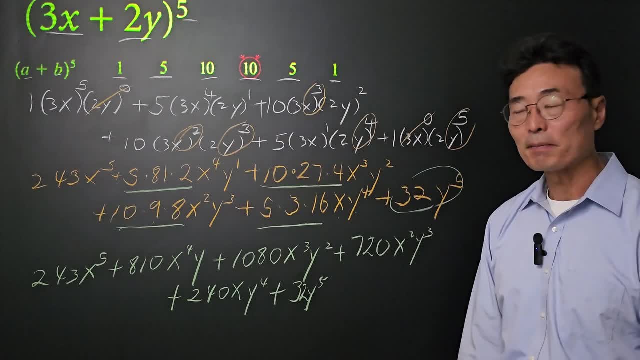 we can do 90 times or we have a 12otto power. So that's always good, but that's a 4 served constant. As you can see, taking the 3x plus 2y to the fifth power doesn't have to be as complicated. 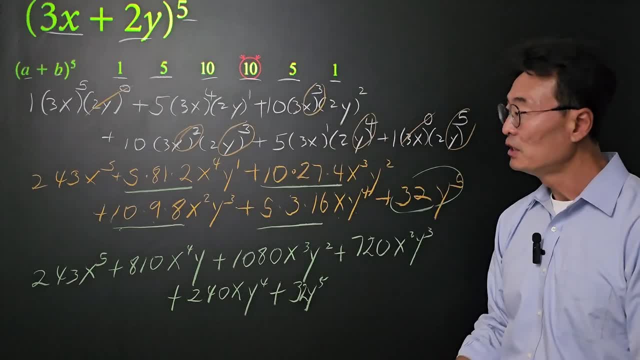 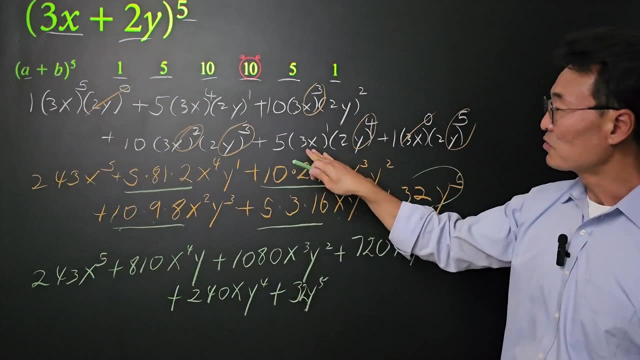 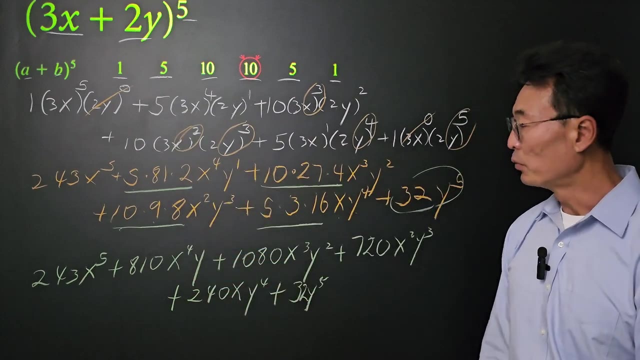 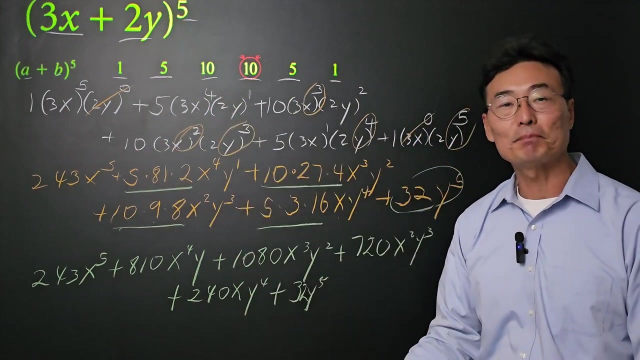 as if you were to multiply them out five times. Rather, if you were to use the Pascal triangle for the coefficients of each term and just take care of the coefficient to the power, then the problem can be solved without too much headache. Imagine, instead of five, if you had a six, seven or eight power. then the problem becomes. 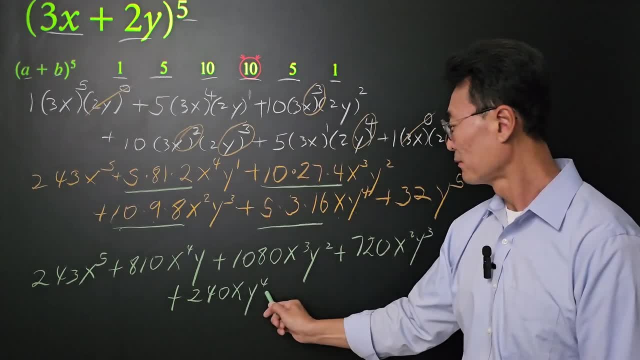 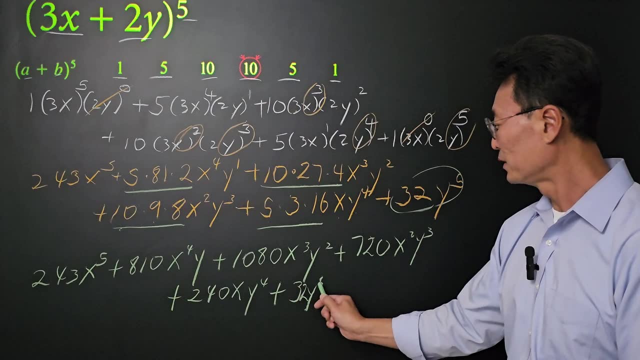 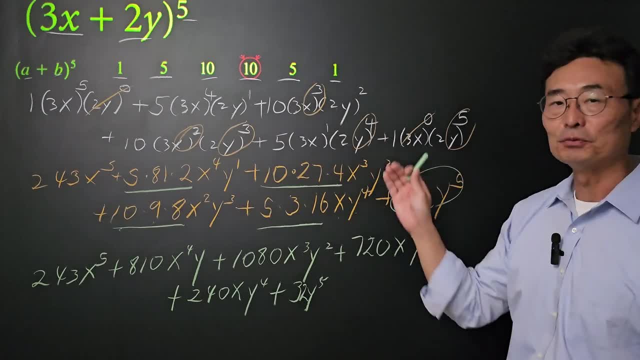 so, as you can see, so, as you can see, taking the 3x plus 2y to the fifth power, taking the 3x plus 2y to the fifth power, taking the 3x plus 2y to the fifth power doesn't have to be. 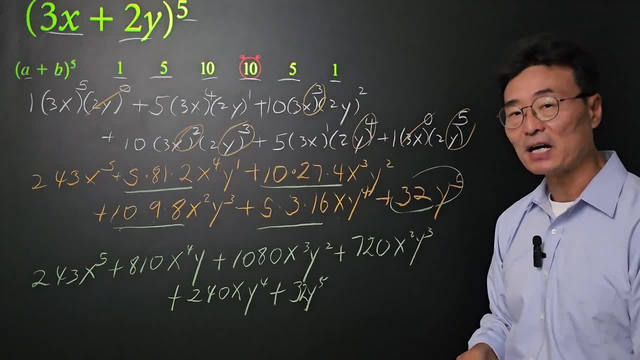 doesn't have to be, doesn't have to be as complicated as if you were to multiply, as complicated as if you were to multiply, as complicated as if you were to multiply them out, them out, them out, five times. rather, if you were to use the five times, rather if you were to use the. 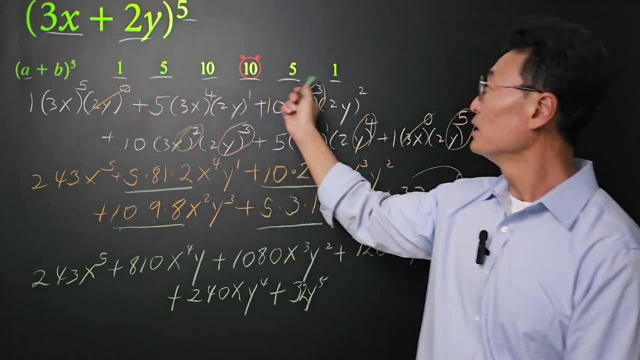 five times, rather, if you were to use the pascal triangle, pascal triangle, pascal triangle for the coefficients of each term, for the coefficients of each term, for the coefficients of each term, and just take care of the and just take care of the and just take care of the coefficient to the power. 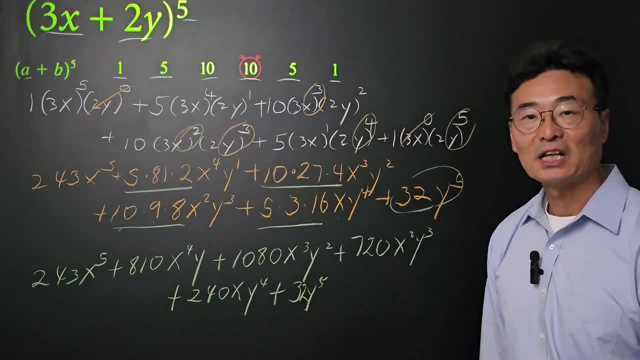 coefficient to the power. coefficient to the power. then the problem can be solved without. then the problem can be solved without. then the problem can be solved without too much headache. imagine instead of too much headache. imagine instead of too much headache. imagine, instead of five, five, five, if you had a six, seven or eight power. 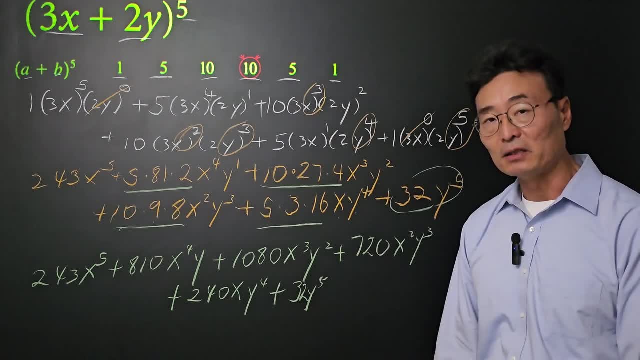 if you had a six, seven or eight power. if you had a six, seven or eight power, then then, then, the problem becomes exponentially greater. the problem becomes exponentially greater. the problem becomes exponentially greater. whereas, if you were to use the pascal, whereas, if you were to use the pascal, 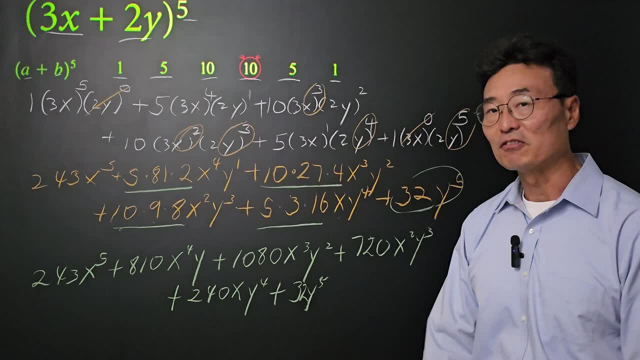 whereas if you were to use the pascal triangle for triangle, for triangle, for the coefficients, it's not as bad, and of the coefficients, it's not as bad, and of the coefficients, it's not as bad. and, of course, course, course. rather than using the pascal triangle, you. 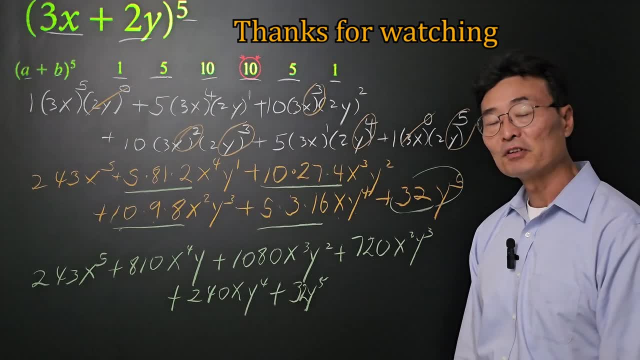 rather than using the pascal triangle, you rather than using the pascal triangle you. i hope you enjoyed this video on. i hope you enjoyed this video on. i hope you enjoyed this video on expanding binomial using pascal triangle. expanding binomial using pascal triangle. 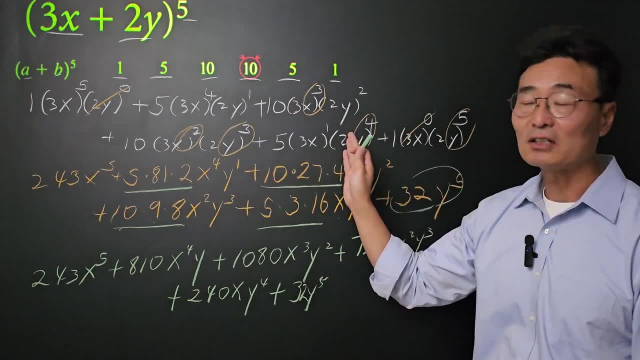 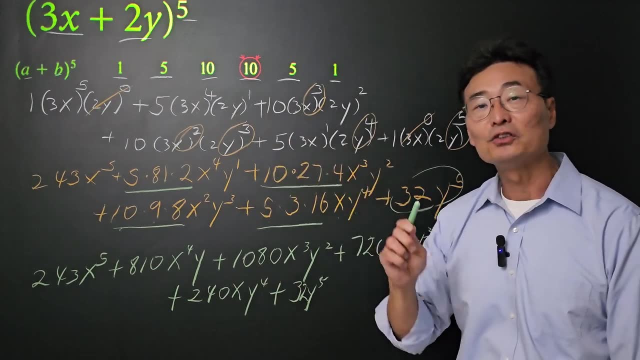 exponentially greater, Whereas if you were to use the Pascal triangle for the coefficients, it's not as bad. And, of course, rather than using the Pascal triangle, you could use the binomial theorem, which I'm going to be going over in another. 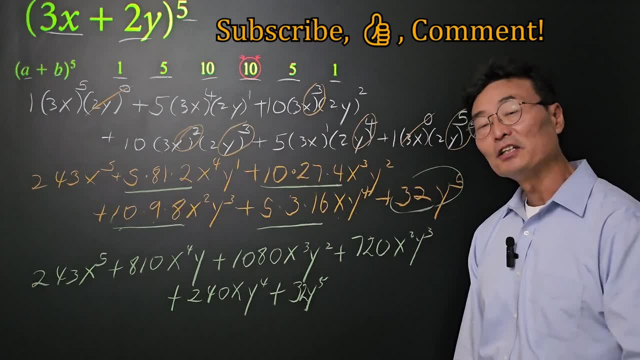 expanding binomial using pascal triangle and hopefully this will be helpful and hopefully this will be helpful and hopefully this will be helpful in your studies, in your studies. 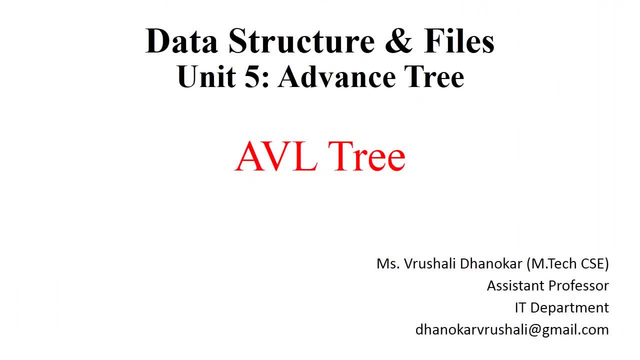 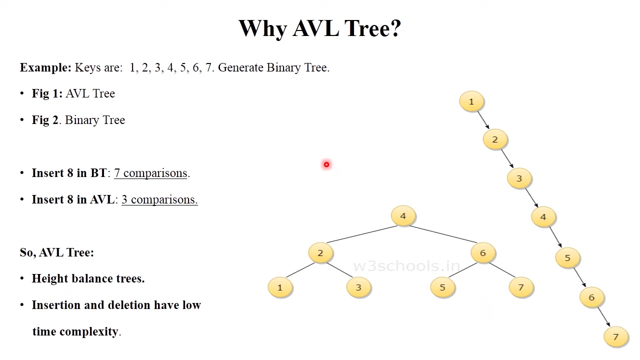 Okay, good morning, And today's topic is AVL tree. In my previous video we learned about red, black binary tree. Okay, and now AVL tree. So let's see what is meant by AVL tree. Okay, so first, why AVL tree? Why we used AVL tree. Okay, see in this example, the given example. 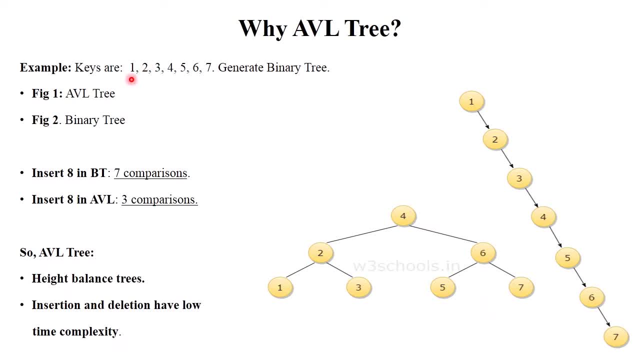 is you need to generate tree. Okay, by using this value: 1,, 2,, 3,, 4,, 5,, 6,, 7.. Okay, so this first figure show AVL tree and second figure show binary tree You all are familiar with.